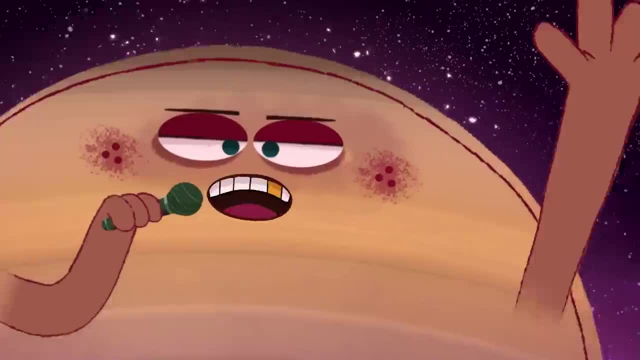 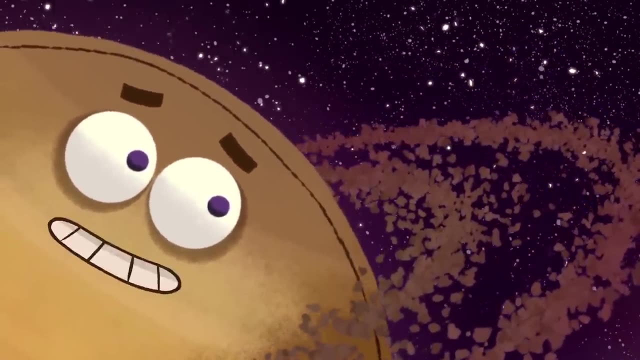 I'm Jupiter, the biggest planet. I'm humongous gargantuan. I spin the fastest, rap the fastest. Plus, I'm handsome, bland son, Oh please. I'm Saturn. Check out my beautiful rings Made up of billions of rocks, dust and other things. 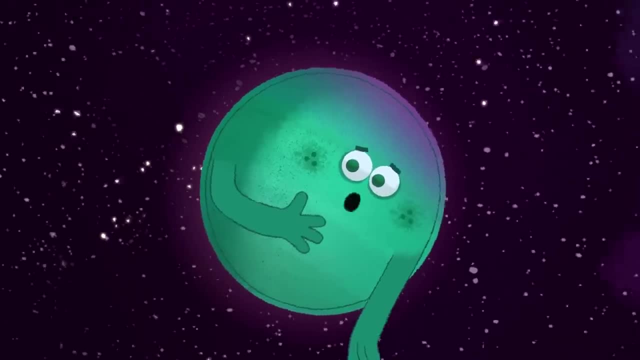 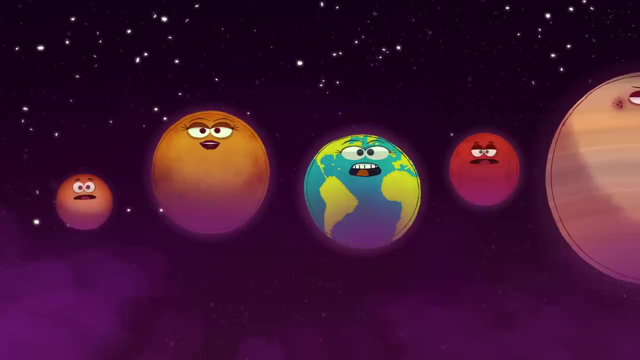 I'm Uranus. I say that with pride. Okay, I lied, I'm embarrassed because I'm the only planet lying on its side. I'm Neptune. I'm cold, dark, windy and mysterious. I'm very stormy, so bring an umbrella. I'm serious. 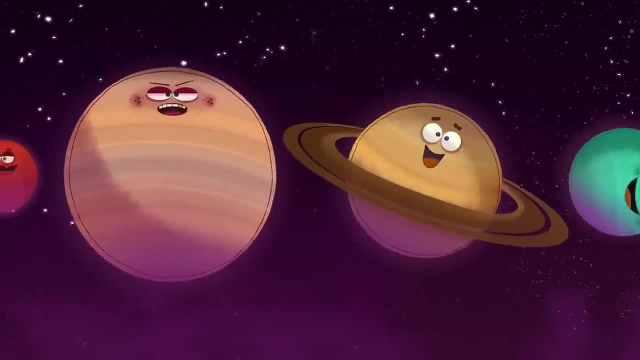 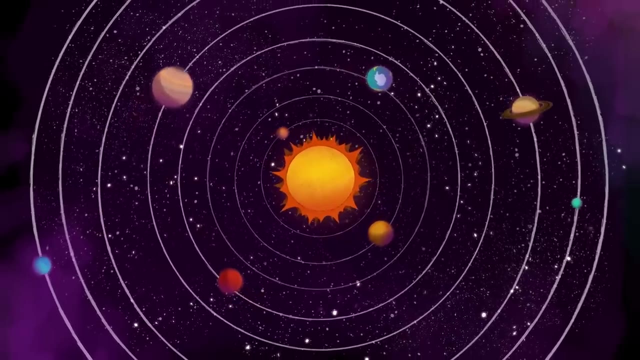 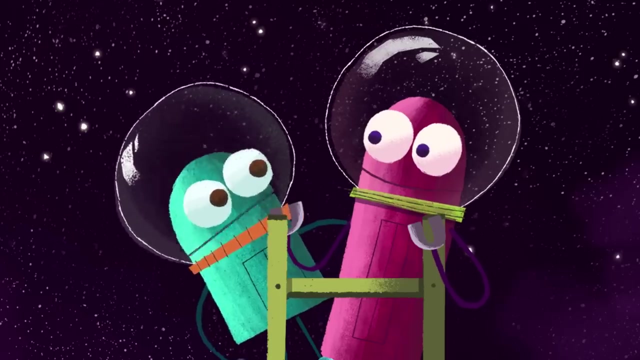 We are the planets of the solar system, Different sizes for everyone. The music never ends. We are such good friends And we all orbit the sun. Well, we are done exploring the solar system. I am thirsty. Let's explore the rest of the Milky Way galaxy. 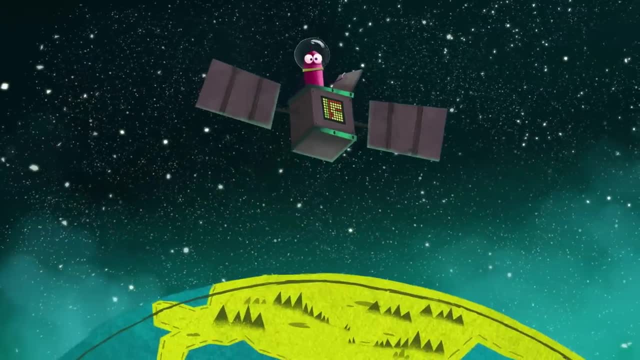 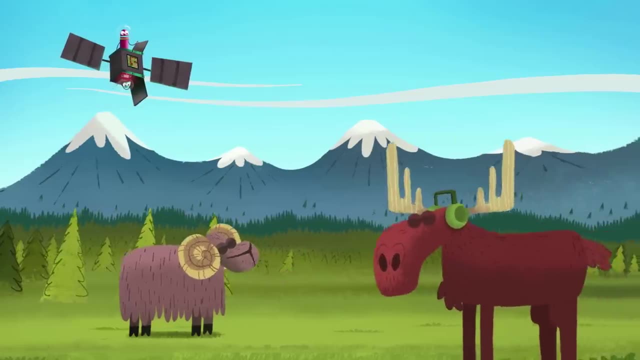 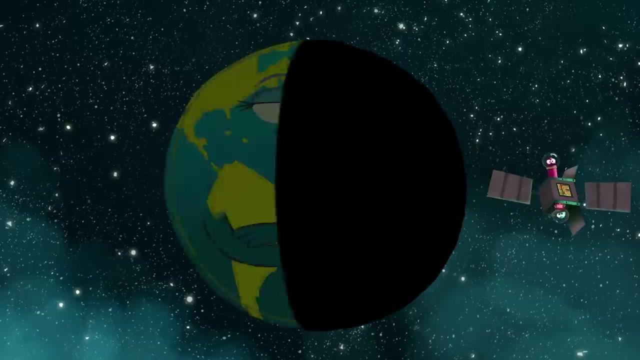 We are currently orbiting planet Earth. I'm picking up some noises, Sounds like cool music, Beautiful, Such a beautiful, Such a beautiful, beautiful world. I'm the earth and for what it's worth, 25,000 miles is my girth. 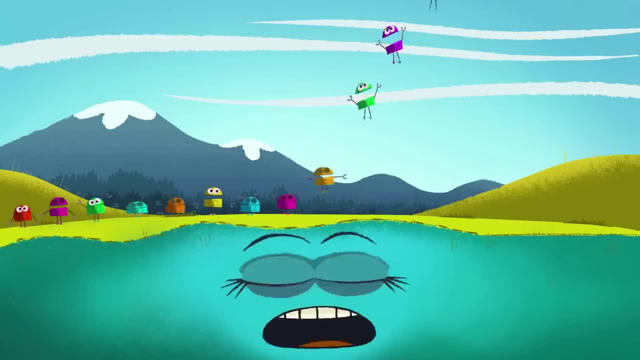 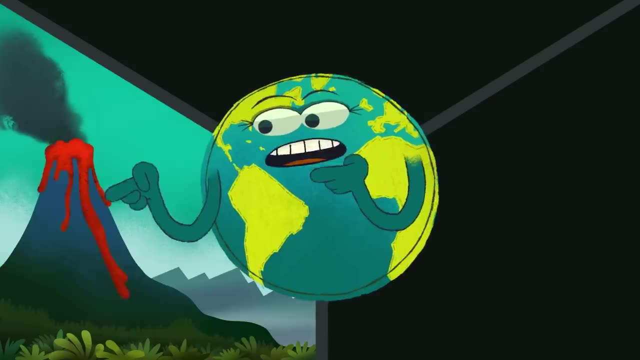 I've got more than 7 billion people living on me all across my amazing geography. Check out my mountains, valleys, trees so tall, and I got lakes, rivers and waterfalls, Volcanoes, craters, swamps with alligators, tropical islands at my equator. 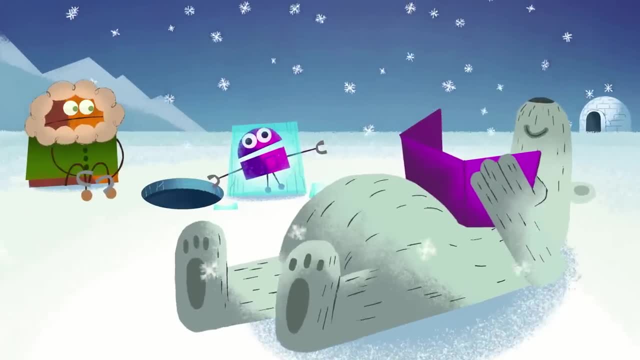 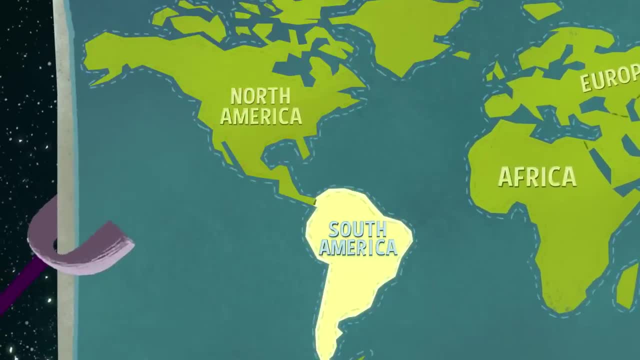 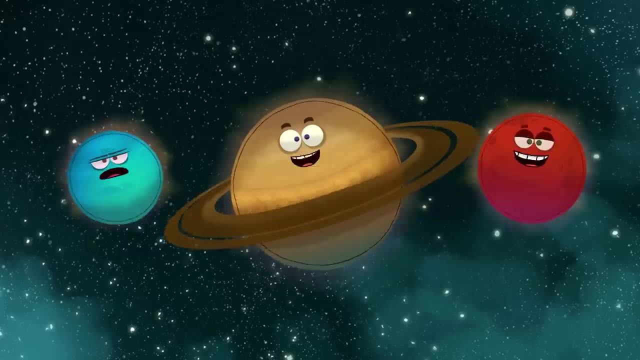 I've got seven. seven different continents- North and South America, Europe, Asia, Africa, Antarctica and Australia- But the biggest thing everybody can see is that I've got a lot of water all over me. I have oceans with lobsters, whales, otters. 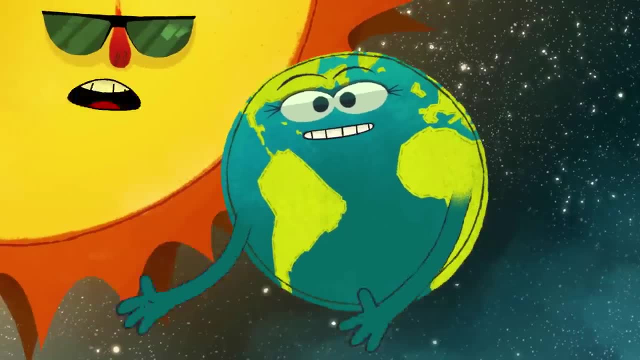 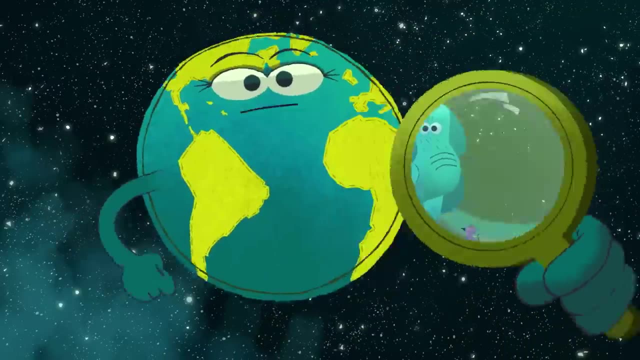 Three-quarters of me is covered in water. I orbit the sun, that's his line, and the moon orbits me. It's my time to shine. I feel it with life, both big and small. the most beautiful planet of all, Such a beautiful, such a beautiful. 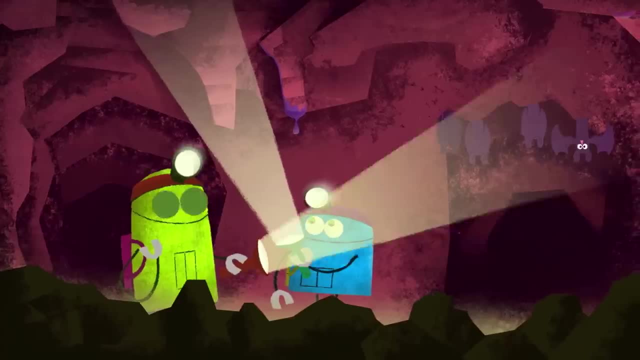 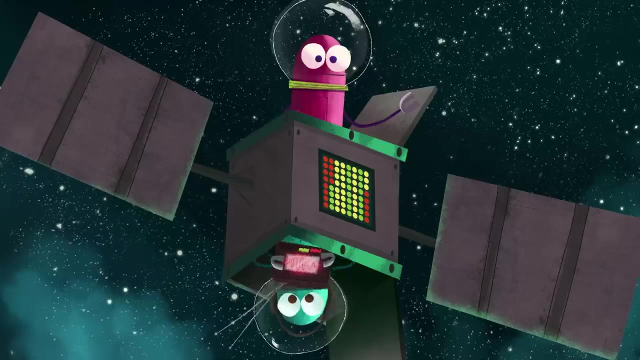 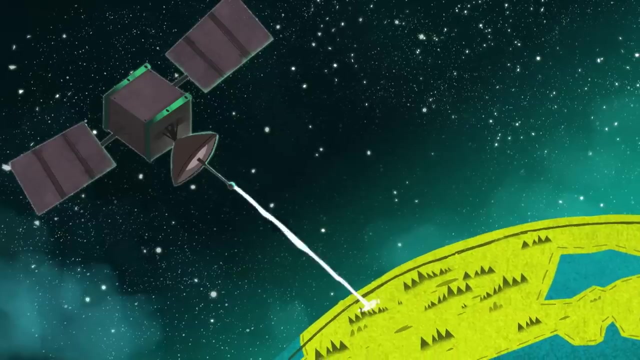 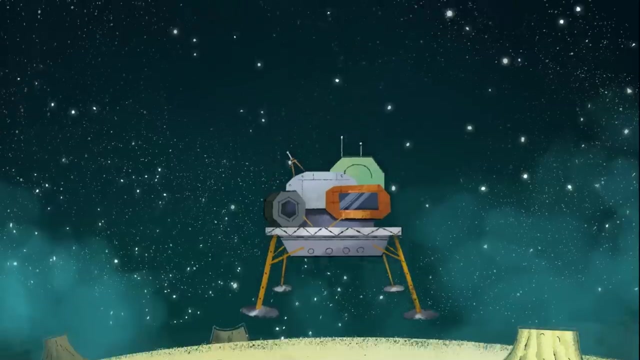 such a beautiful, beautiful world. It is the home to every boy and girl. It's a beautiful, beautiful world. I'm getting homesick, Me too. Computer, take us home Repairing to land our spacecraft on the moon. Houston, we have a song. 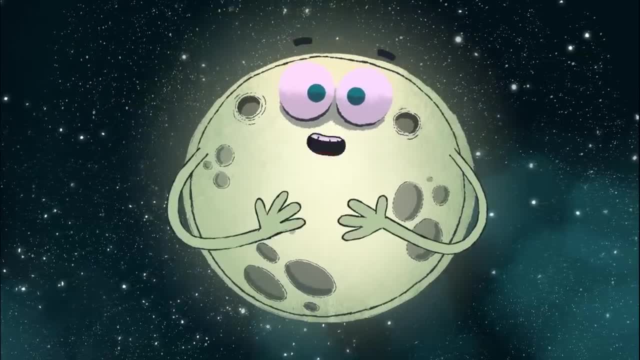 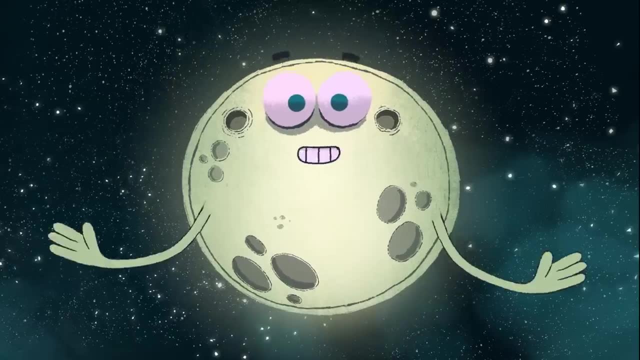 It's my time to shine. It's my time to shine. The day is over now, so it's my time to shine. Good evening, it's the moon here to regale you with a tune. I'm so bright up in the sky at night. 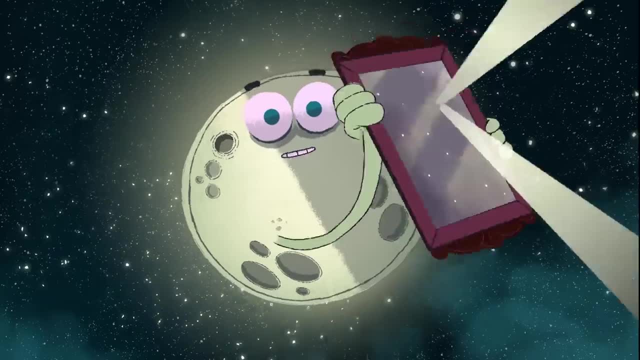 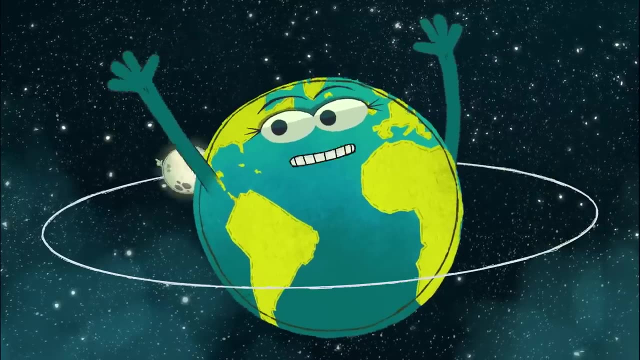 but the truth is I'm just reflecting light. See, let me help you break it down. The Earth and I are spinning around and I orbit the Earth in a loop. You see, the moon is kind of like my hula hoop. 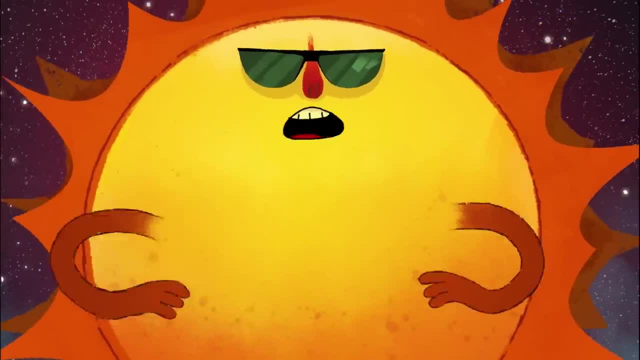 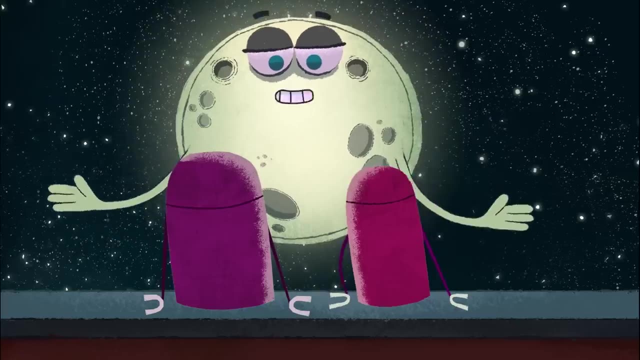 We both orbit the sun. He's the big shot. I'm the center of the solar system. I'm so hot. The sun's like a light bulb and I'm like a mirror. Light bounces off me and then it appears to the Earth below for a lovely view. 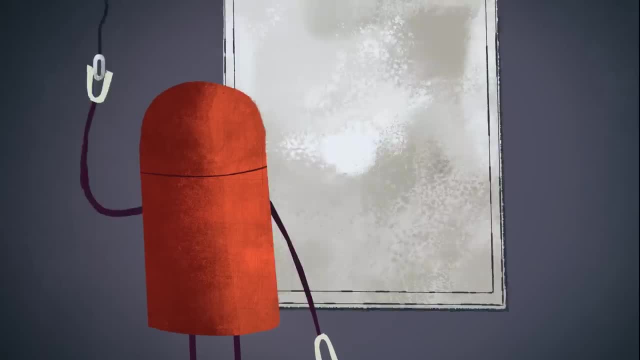 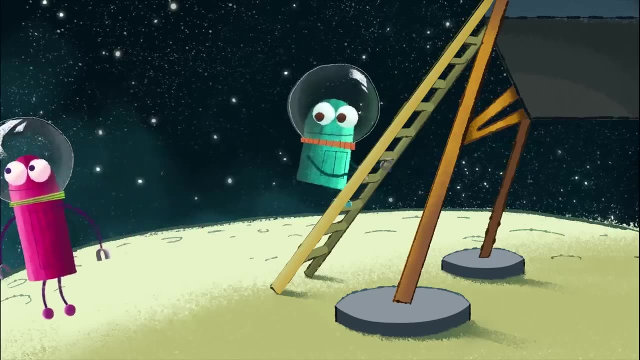 for animals like wolves who go awoo. Sometimes I'm full, sometimes half on, Sometimes I'm crescent or it looks like I'm gone. But I'm here in the dark, just a lonely moon, hoping that somebody will visit me soon. 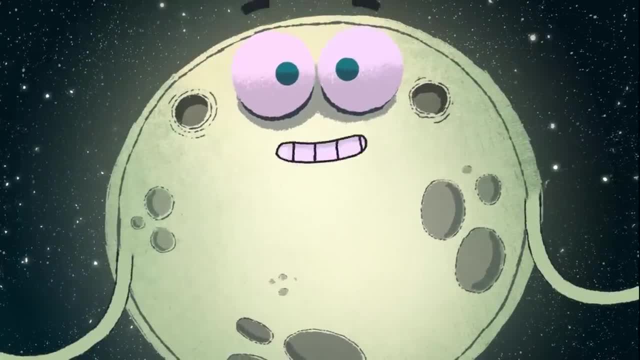 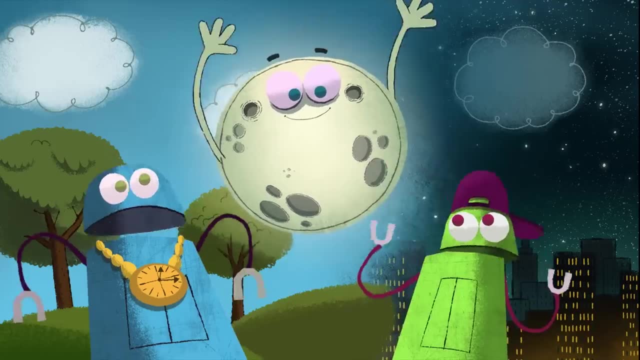 I'm covered in dust and I'm made of rock, So come see me soon and go on a moonwalk. It's my time to shine. It's my time to shine Both at night and at night we can see the moon shine. 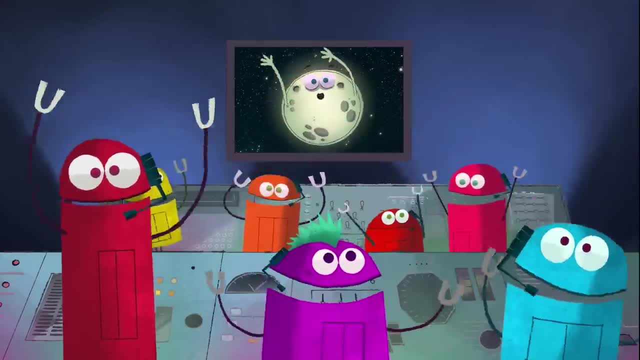 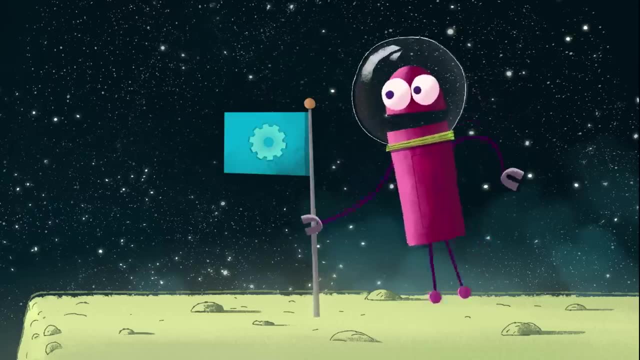 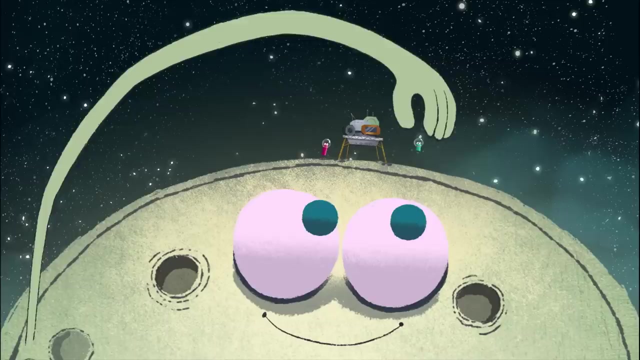 It's my time to shine. It's my time to shine. I'm planting this flag on the mountain I climbed. One small step for a story bot. One giant leap for story bot kind. One giant leap for story bot kind. This is holy. 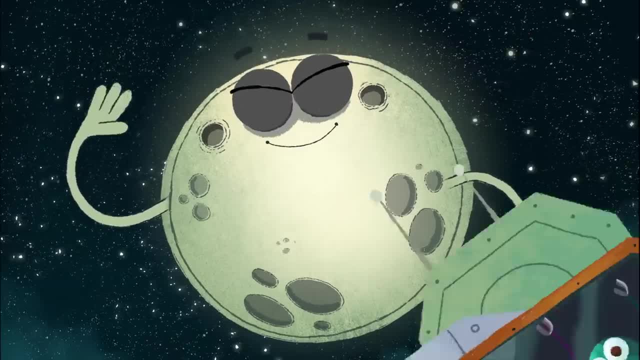 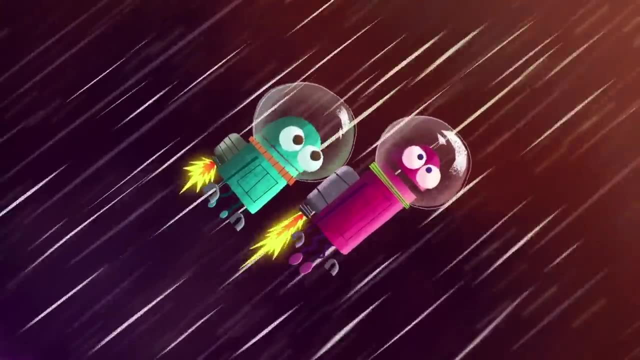 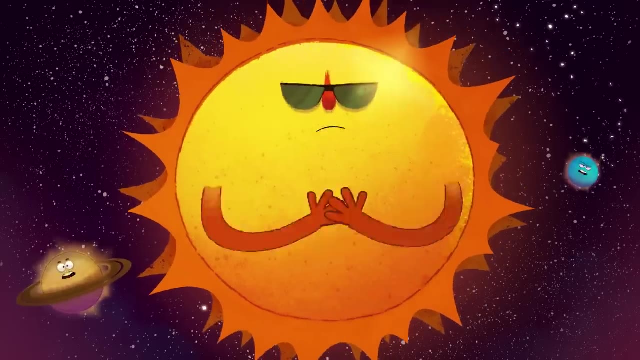 Is this a dream? A dream? It's not a dream, Slow down, It's a reality, something that's just too great. According to my calculations, we are now approaching the sun. It's getting pretty hot in here. I'm so hot. 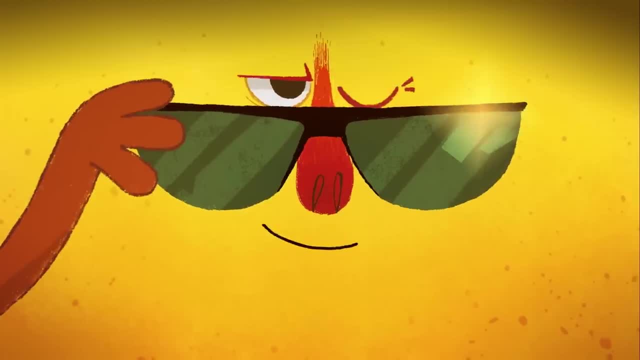 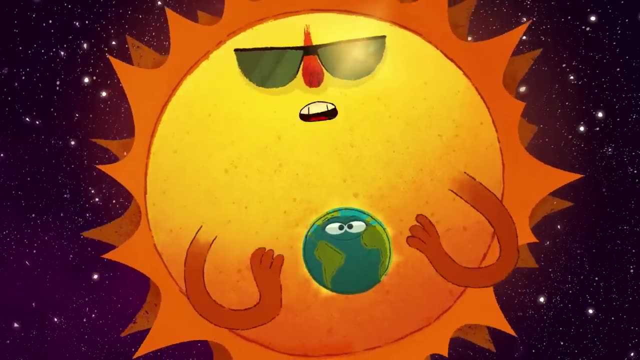 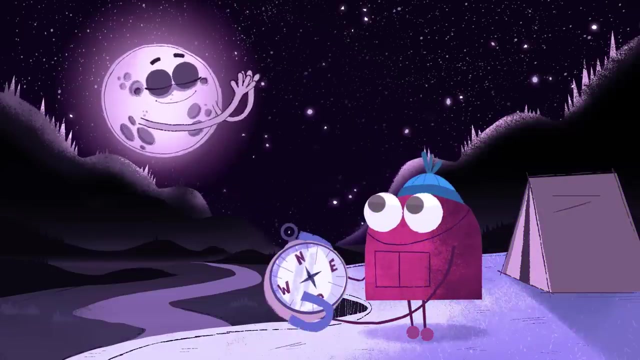 I'm so hot, Check me out. check me out, I'm hot. Yo everyone. I'm the sun 0 of gas like hydrogen and helium. i keep the earth warm and help to grow food. i shine on the beach, on guys who say i set into the west and on comes night, and then i rise from the east with that. 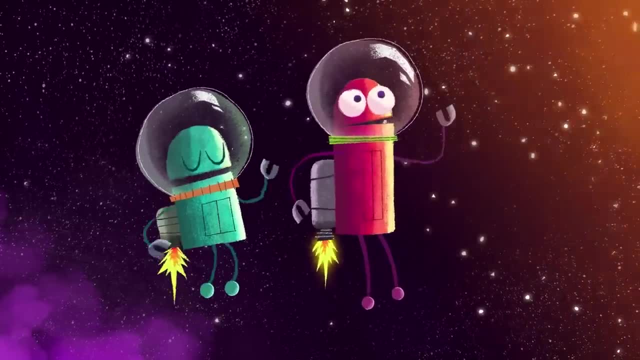 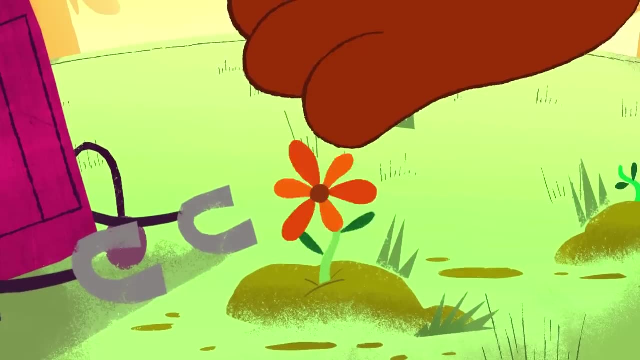 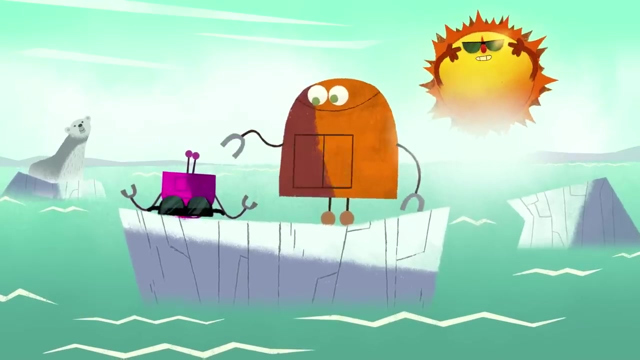 golden light. i'm so hot. so hot and bright, 28 million degrees fahrenheit. i make plants grow like trees and flowers. so powerful got that solar power. make the deserts dry, make the oceans rise. don't stare right at me, i could hurt your eyes. i'm just about a million miles wide. i'm so big. 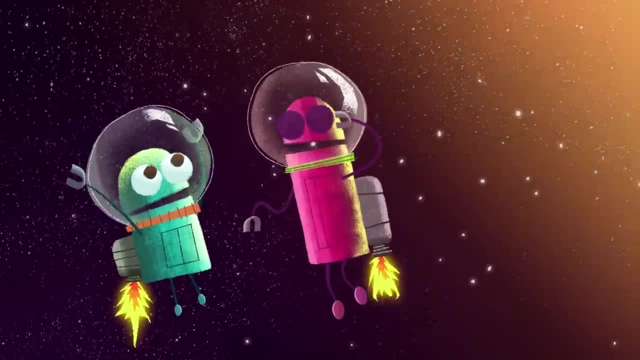 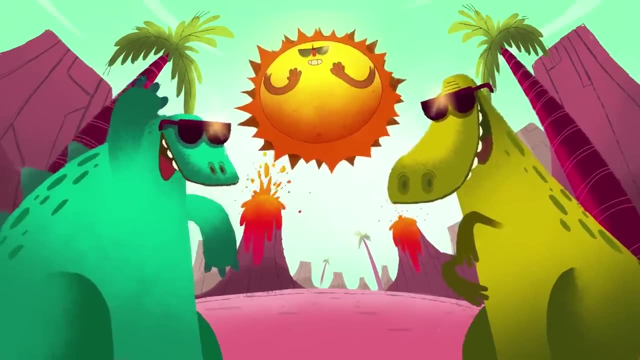 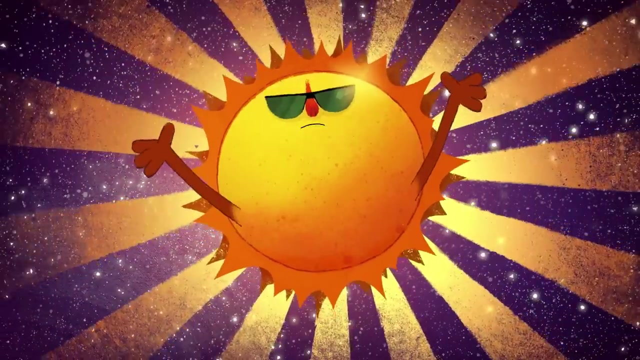 you could fit a million earths inside. i'm the center of the solar system, can't you see? got so much gravity. planets orbit me. i'm four and a half billion years old. in spanish, everybody calls me soul. when i'm not around, you'll be feeling cold. yeah, i shine so bright with my rays of gold. 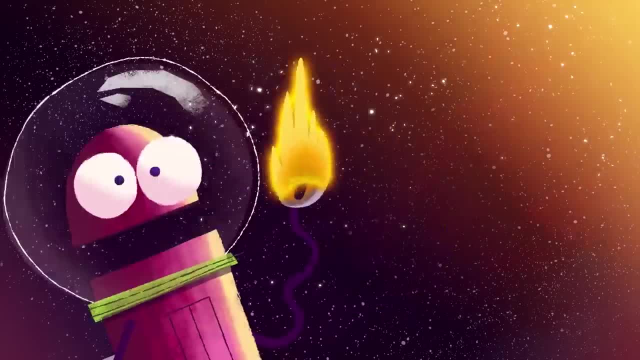 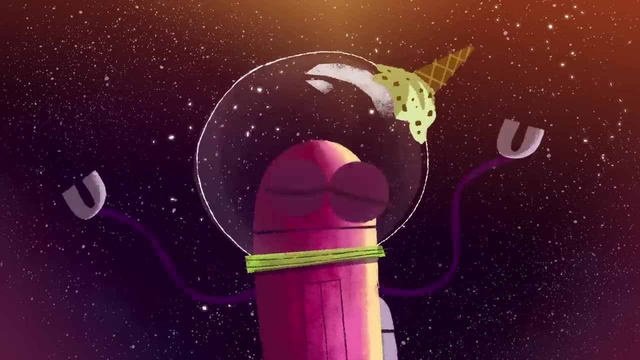 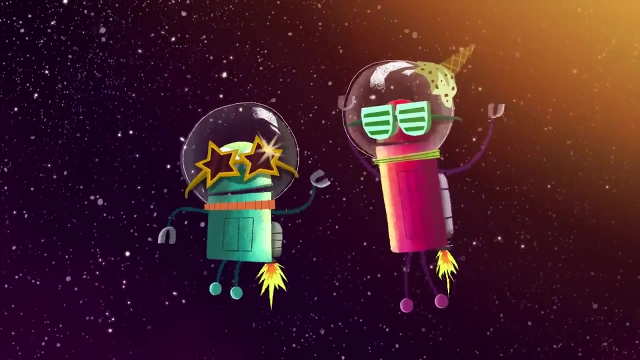 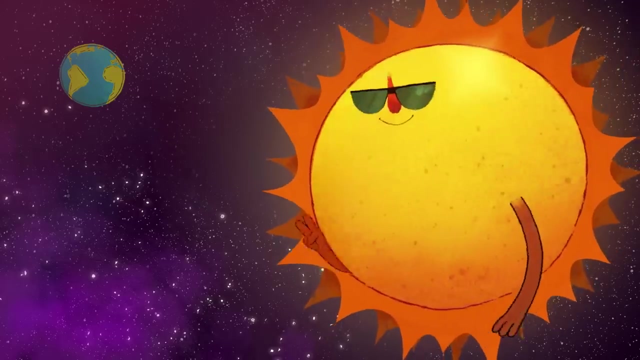 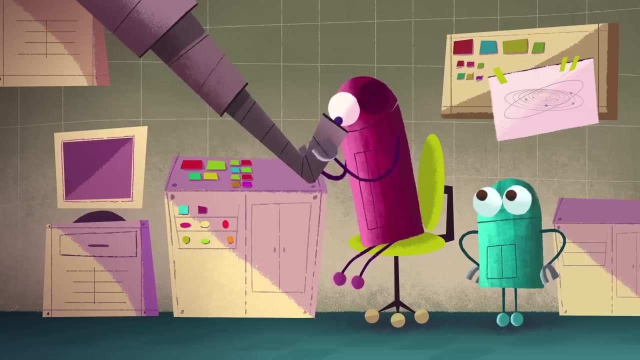 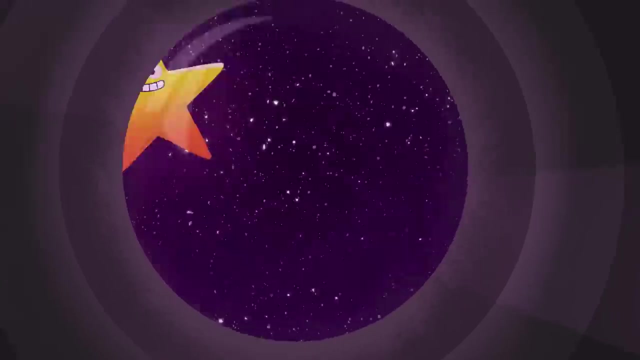 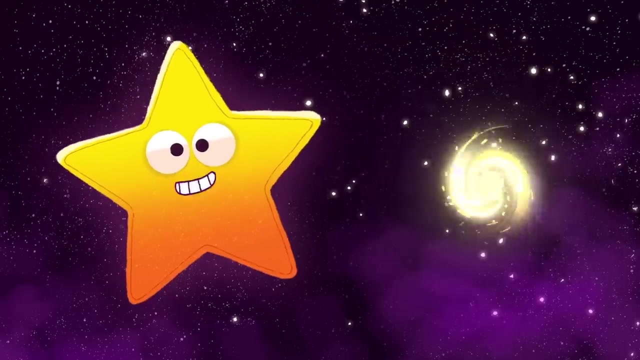 i'm so hot. i'm so hot. oh, he's right, he's. come on, storybots, show me what you got. how hot am i? do you see anything? stars are out tonight. i'm a star. i'm a star from afar, yes, you are. so am i here? balls of hot gas that shine in the sky there. 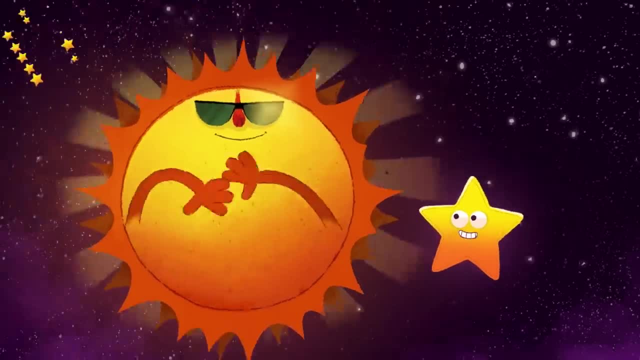 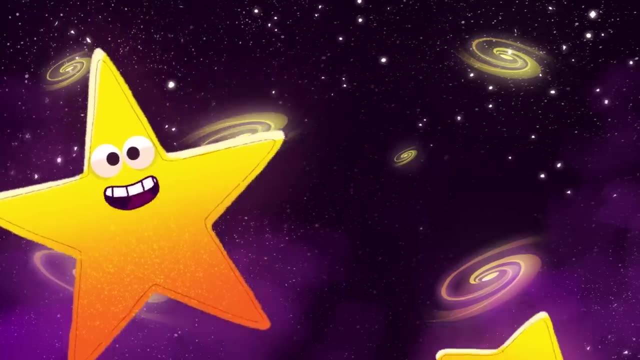 are trillions and trillions of us. that's a lot. even the sun is a star. there are lots of other stars like him and me and a bunch of us together form a galaxy. there's billions of galaxies, lots of stars understand. there's more stars in space and all of earth's grains of sand from land with. 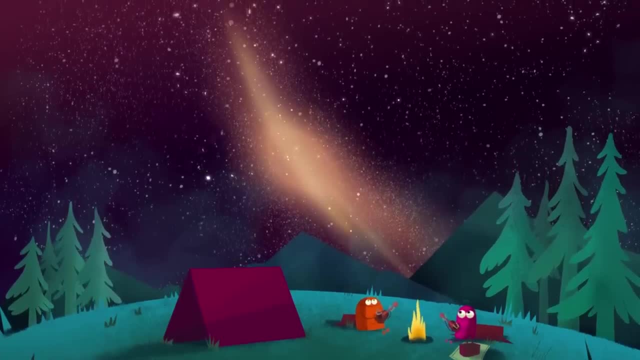 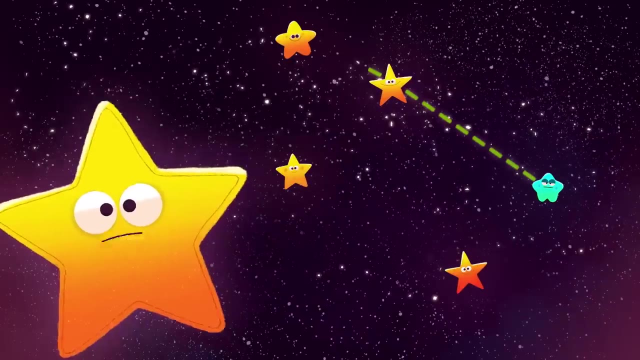 your eye to the night sky display, you can see the earth's sky, and you can see the earth's sky and the earth's galaxy, the milky way. stars are different sizes and we can more. there are super giants, giants and dwarfs, and we form constellations which are patterns of stars, the four gps. that's how. 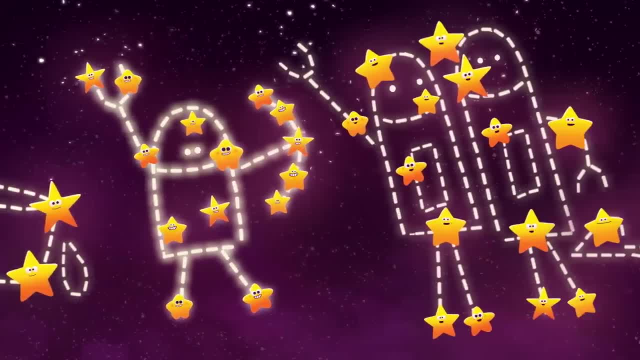 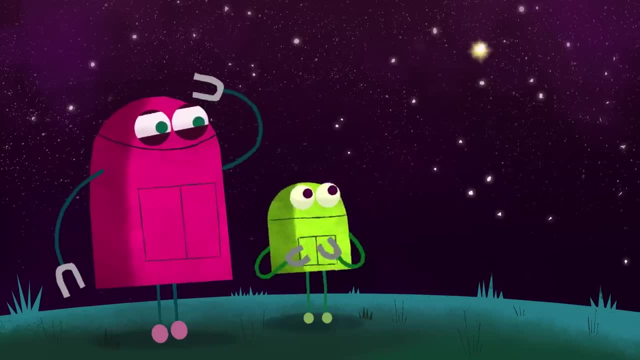 you know where you are. we're the big dipper. we're the belt of the right. we're the gemini twins. people think we twinkle, but that's not true. the light's just playing tricks when it shines on you. and shooting stars aren't stars. no, they're not. they're meteors burning up when they get too hot. 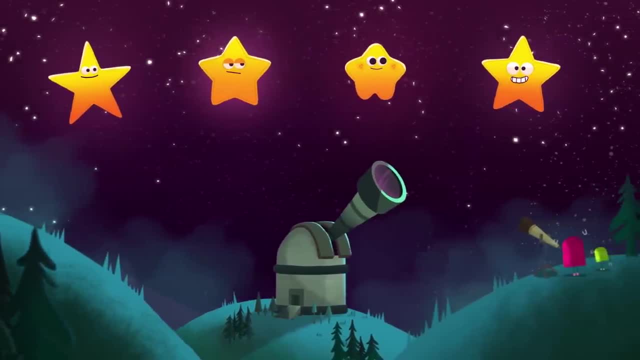 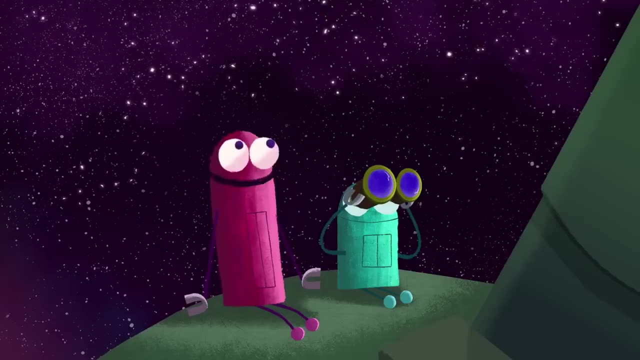 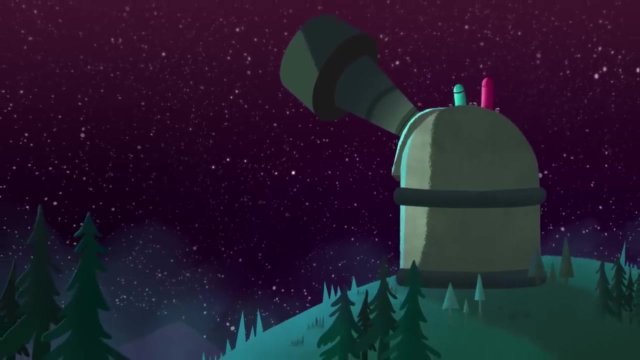 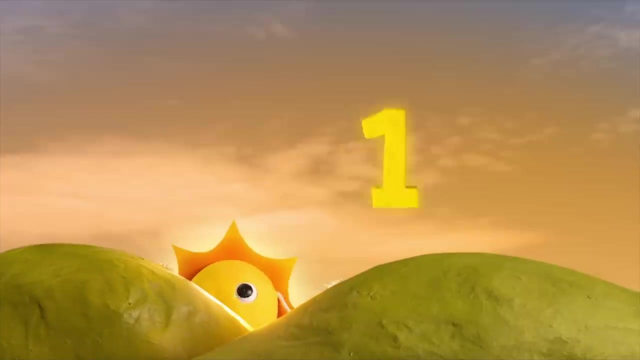 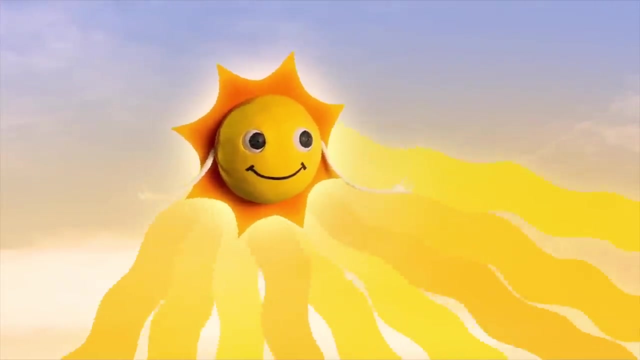 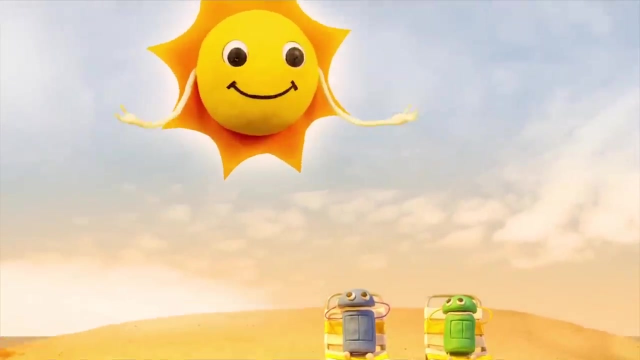 wish upon a star might come true, you know, i hope. look up in the night sky or look through a telescope. that's true, there really are. i made a wish. what was it? i'm not telling. one, two, one, two, three. let the day go and everything shines bright. 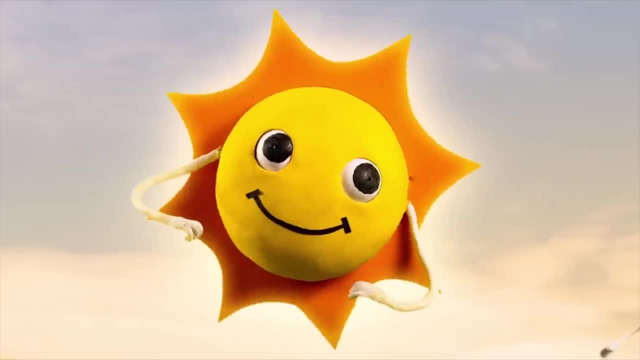 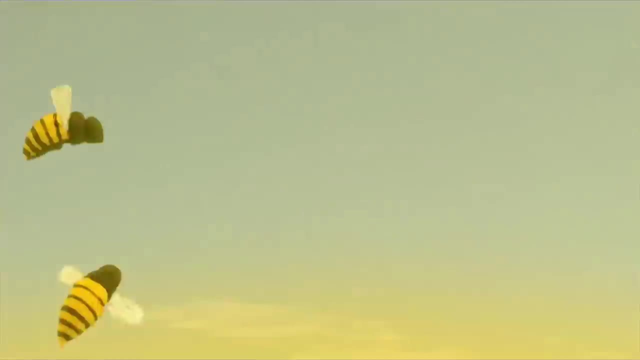 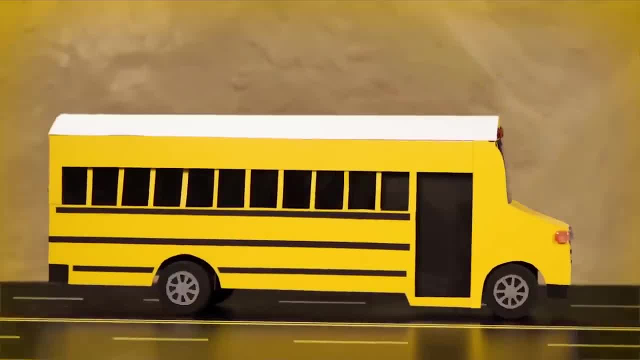 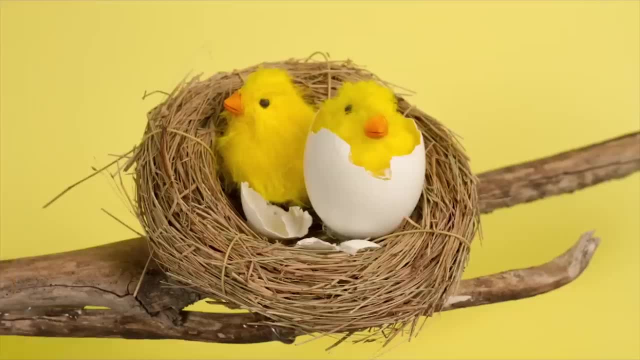 Bananas, don't forget to peel Cheesy macaroni. or a big school bus. Yeah, it means slow down, even when you're in a rush. There's yellow buttercups- how could I forget Color of canaries- and little baby chicks- Summertime trips: put that in the mix. Yellow means happy. it feels like this. 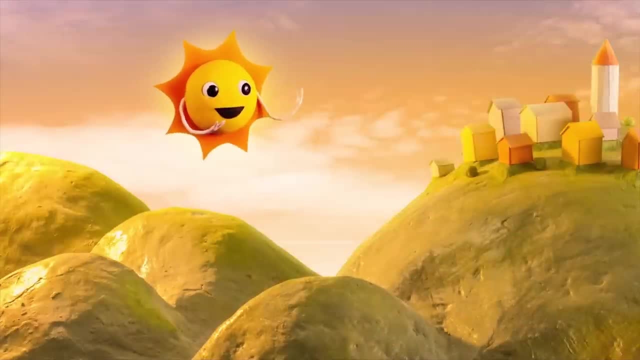 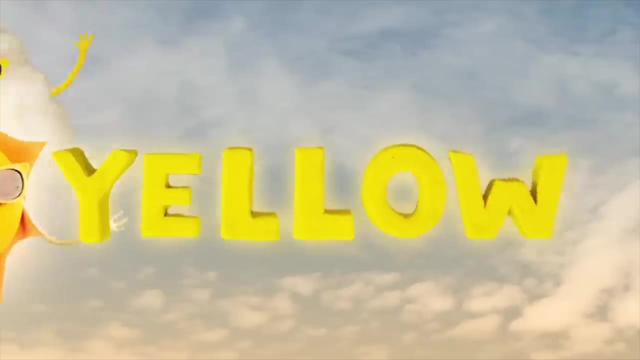 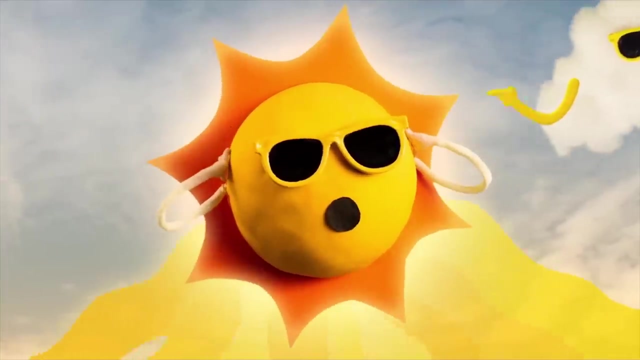 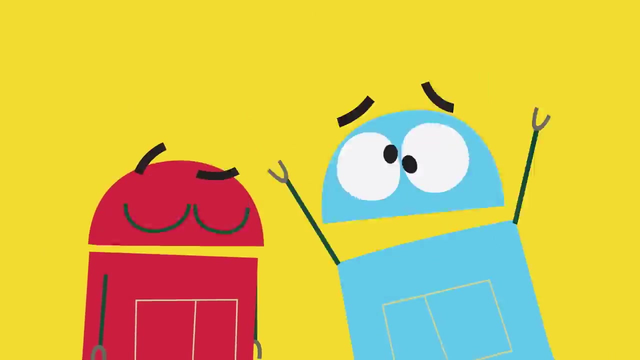 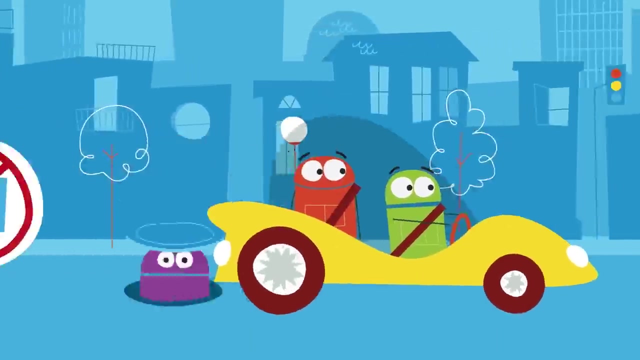 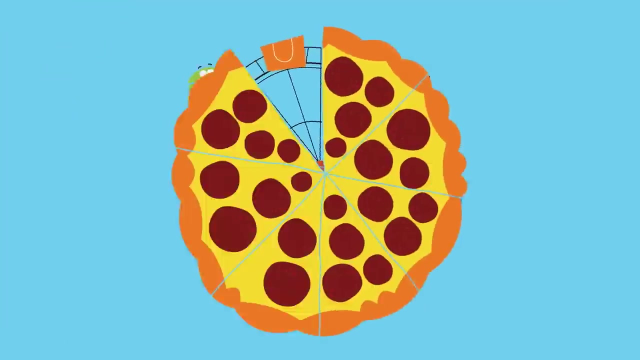 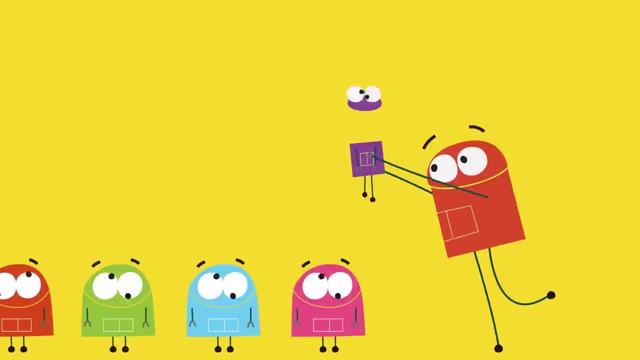 Sunlight. let the day go When everything shines bright And we'll take the day slow. Sunshine is yellow Pizza pie. take a look at those googly eyes. Googly, googly, googly, googly eyes, Googly eyes, yeah, yeah, yeah, yeah. Circles a quarter circles a trash can lid. 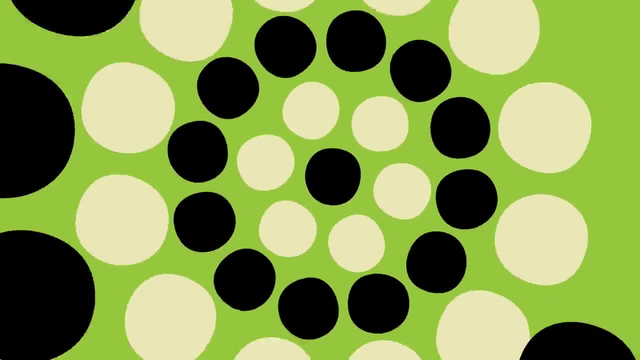 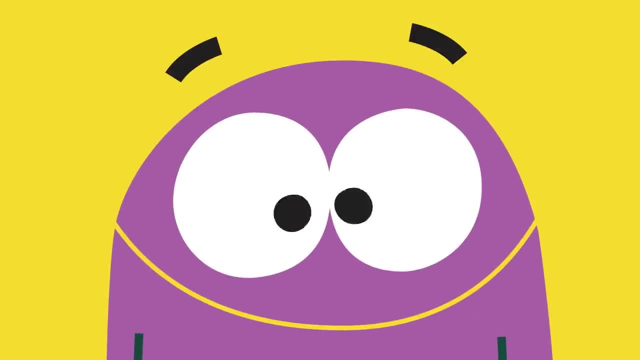 Circles, a record on a record player. Circles going round and round, A soccer ball and a smiley face, A button, a clock, pancakes, Bicycle tie- let's go for a ride. Take another look at those googly eyes. Googly, googly, googly, googly eyes. We've got googly eyes. 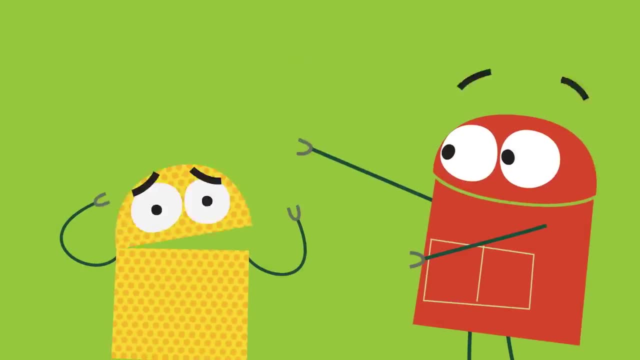 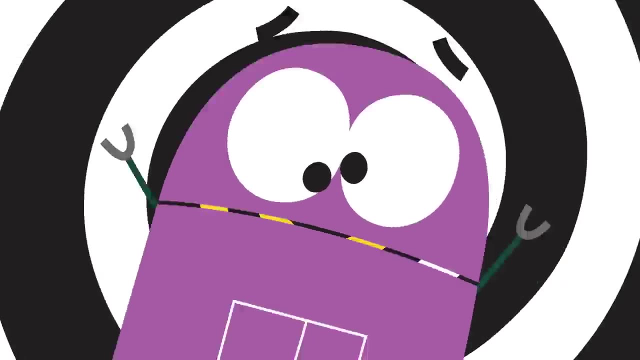 Yeah, yeah, yeah, yeah. Circles All over the place, Circles Right on my face, Circles All over town, Circles going round and round, Just like googly eyes. Circles going round and round and round. Who's got googly eyes? 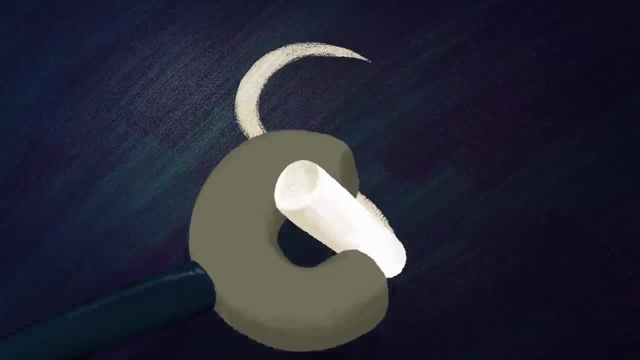 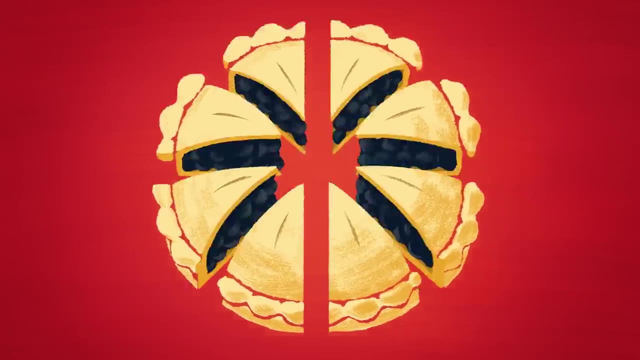 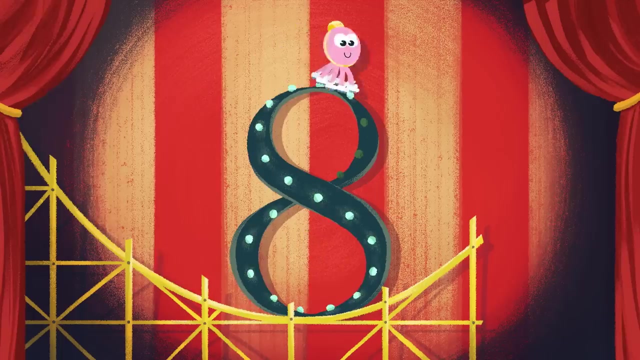 We do. Number eight has kept me smiling since I learned to count that high. I always cut eight slices when I serve a piece of pie. I got an octopus named Speedy. She likes to wear eight roller skates. Yeah, When it comes to nifty numbers, You know I love those crazy eights. 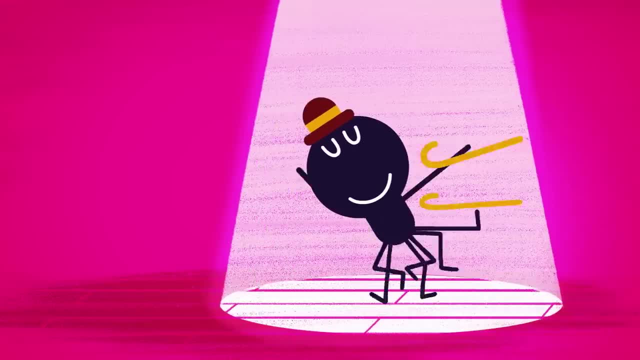 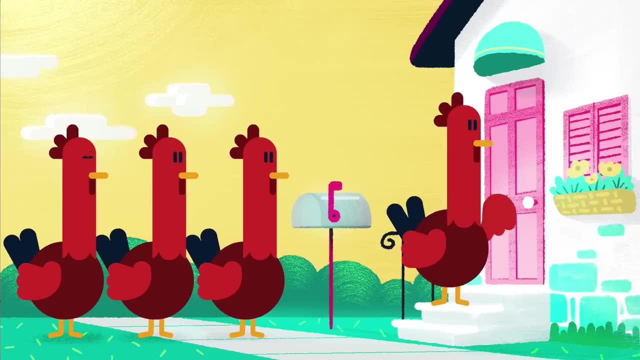 One, two, three, four, five, six, seven, eight. I count eight legs on a spider. A stop sign's got eight sides. When eight hippos hit the playground at games Eight busted slides, Eight chickens have a party. When four roosters bring their dates. 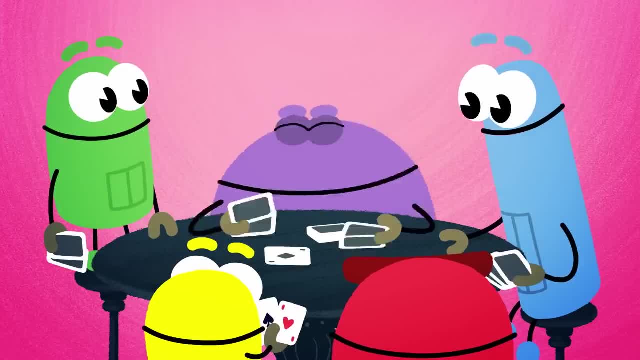 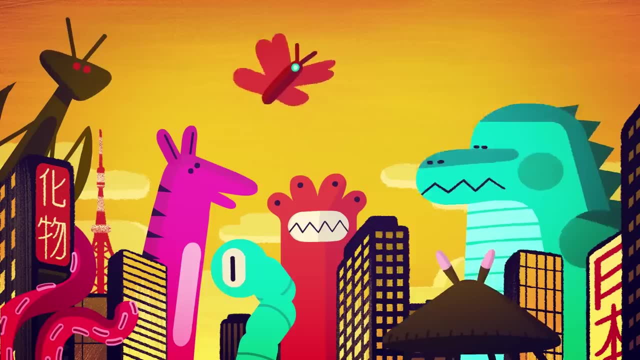 And when it's time for a card game, My favorite one is crazy eights. One, two, three, four, five, six, seven, eight- I can count eight flying saucers, Eight monsters from Japan And eight tigers on vacation in an eight-seat minivan. 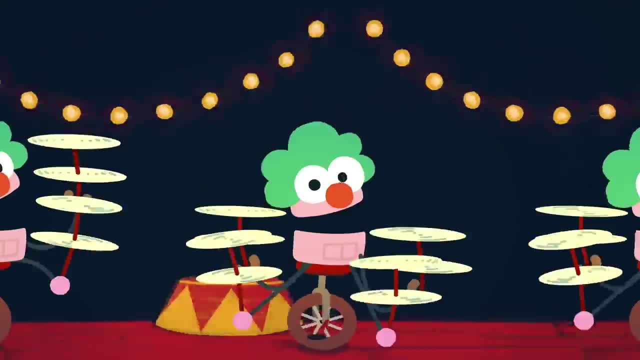 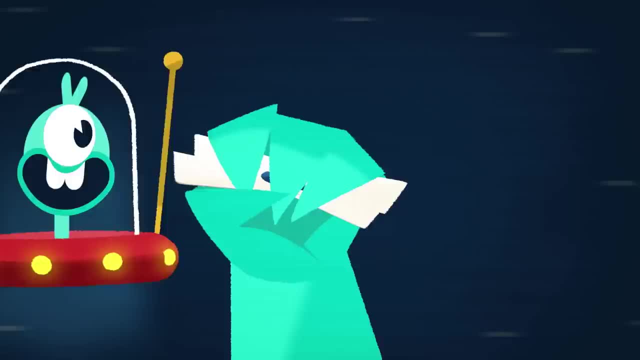 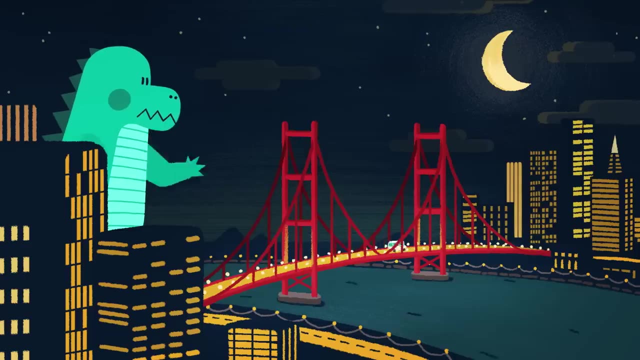 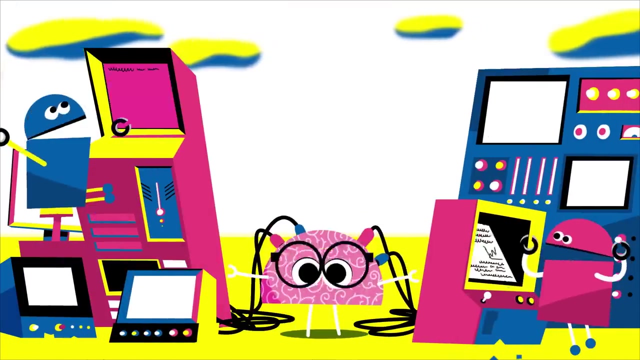 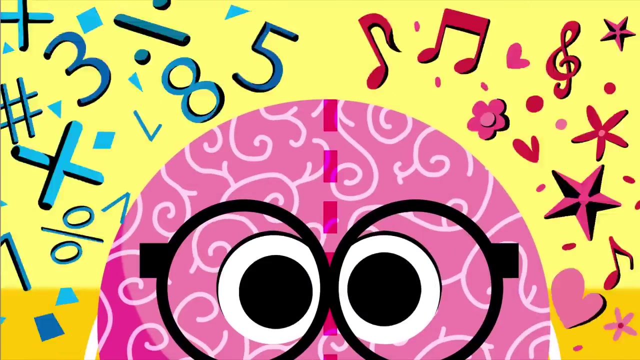 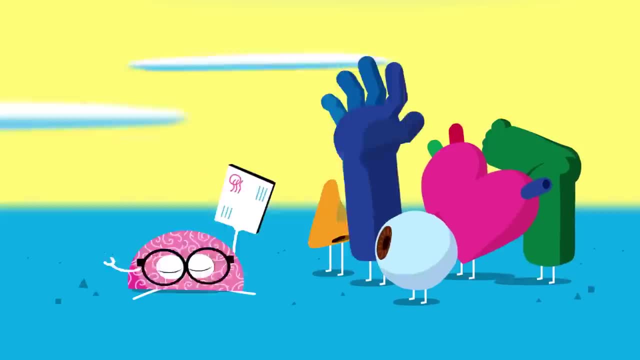 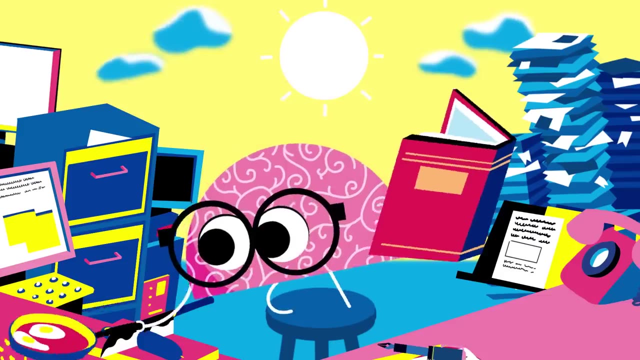